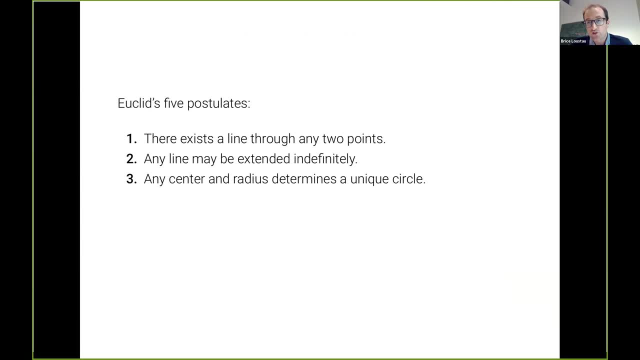 So lines are infinite. One can always draw a unique circle. given a center and the radius, All right angles are congruent, which means they look the same. And finally there's this controversial fifth axiom. that sounds a little more complicated, So let me just show you a picture. 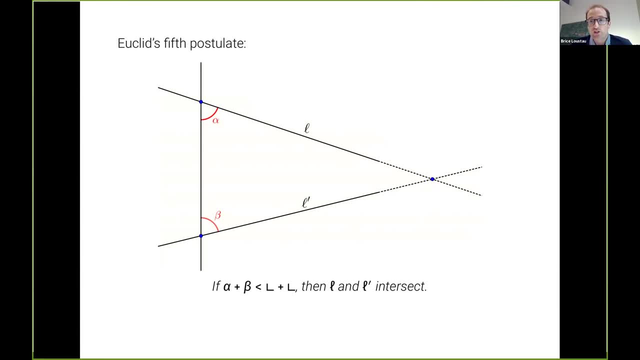 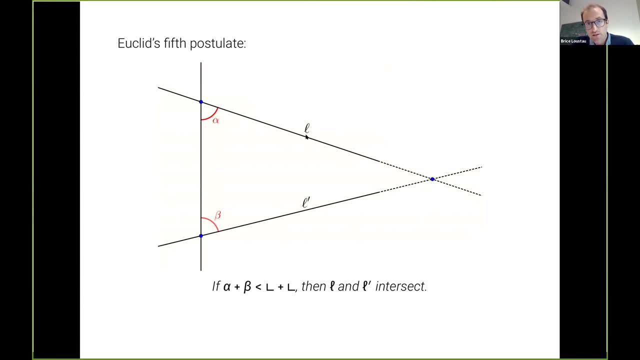 these angles are less than right angles, as on this picture, then these two lines, l and l prime, must intersect. so you might wonder: why is this controversial? it sounds very reasonable, as this picture shows, that l and l prime intersects on the right hand side here, but this seems like it's a little too complicated to be to be a postulated we should be able to. 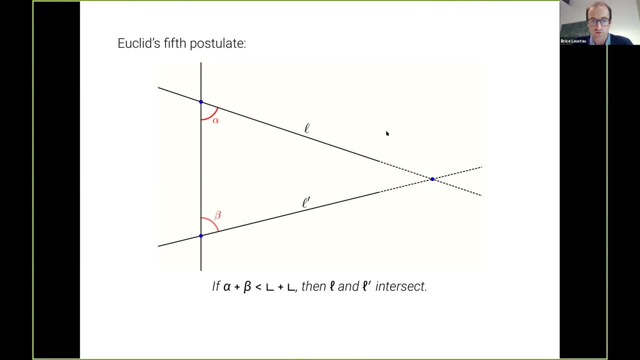 prove this? it shouldn't be one of the most basic truths? and so for. for a long time, mathematicians tried to, to, to derive this axiom from the other form, and they were unsuccessful for almost over 2 000 years. and finally, in the 19th century, mathematicians created or discovered, 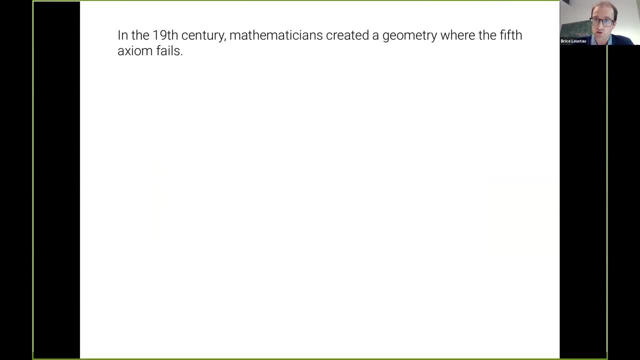 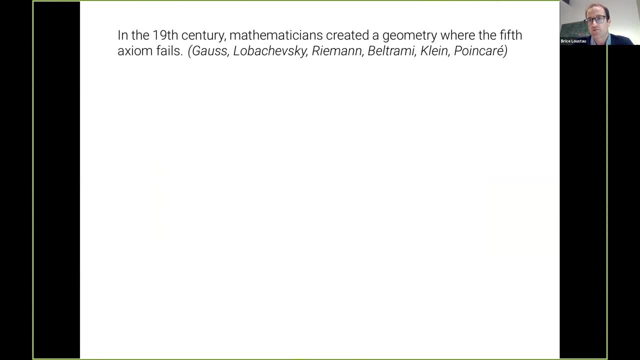 but not the fifth, and this is hyperbolic geometry, and we have some of the most famous mathematician here, who, whose, whose names are attached to this new geometry. so i i want to show you what it is, and there is different models for hyperbolic geometry, but one of the reasons it took so long, 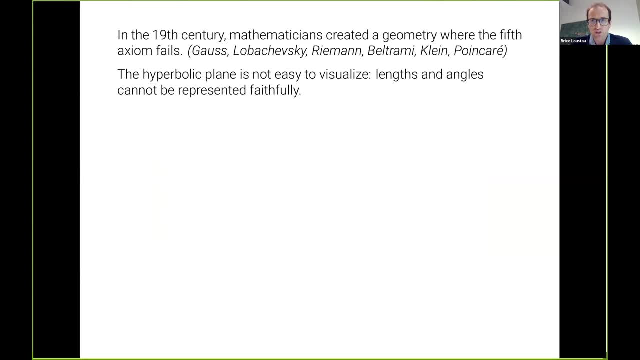 for mathematicians to discover it is that it, unlike spherical geometry, it's hard to represent because there is no perfect way to represent the hyperbolic geometry plane. So this is one of the possible representations of it. is this disk called this the Poincaré disk? So it's the inside of the circle and what we call straight lines in 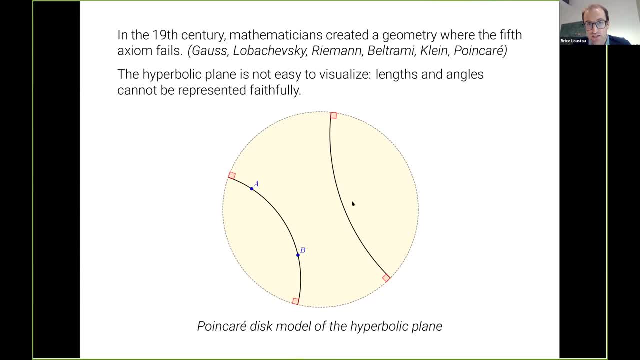 hyperbolic geometry would be these arcs that you see, that are actually arcs of circles, Euclidean circles that are orthogonal to the boundary of the disk. And well, maybe it's, maybe it's kind of clear, for instance, that the first axiom is satisfied. so if I have two points, a and b, I can draw a unique, a unique line, straight line between quotes. 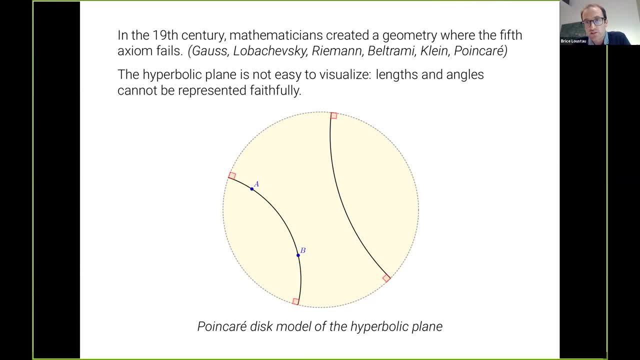 like this. Now, what's what's not accurate in this model is the measurement of distances, because so I would have to tell you what: how you measure hyperbolic distance between points, but it's very different from the Euclidean measurement and, in particular, when you approach. 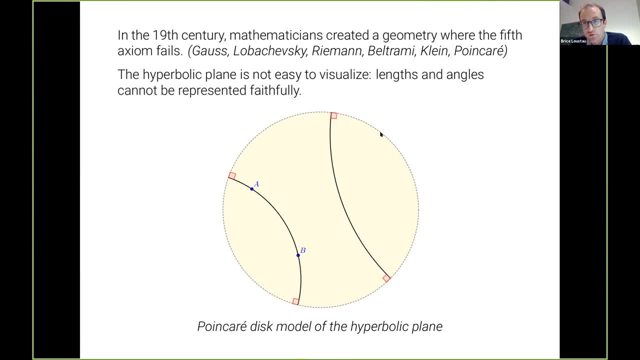 the boundary of this disk, the hyperbolic distance actually explodes. So so this, this hyperbolic disk, looks finite for us, but it's actually infinite for hyperbolic geometry. So I'm going to tell you about another model in in the moment. 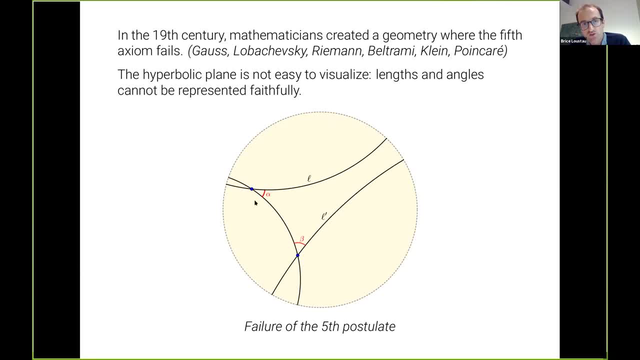 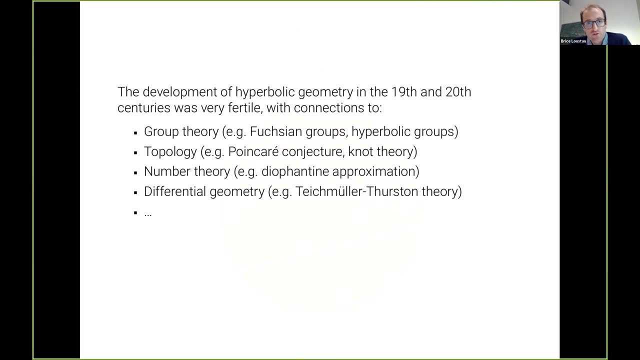 And so here I'm illustrating the failure of the fifth postulate, where you see two lines, L and L prime, that do not intersect, even though those angles- alpha and beta- are less than 90 degrees. So the development of hyperbolic geometry in the 19th and 20th century was: 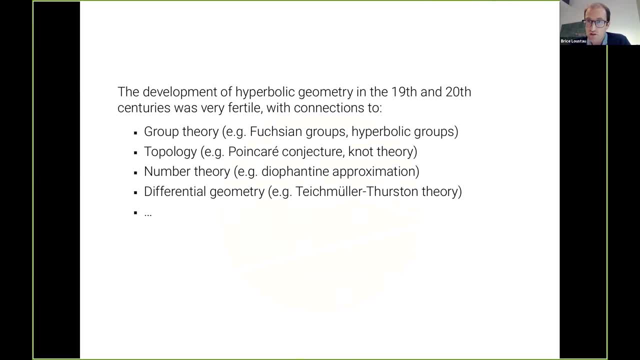 incredibly fertile, with many applications, both in pure and applying mathematics and other sciences. So so here I just listed a few. you know that I could talk about for a long time, but today I want to focus on two particular connections, which is the theory of relativity and and data science, And so I'm going to tell you more about. 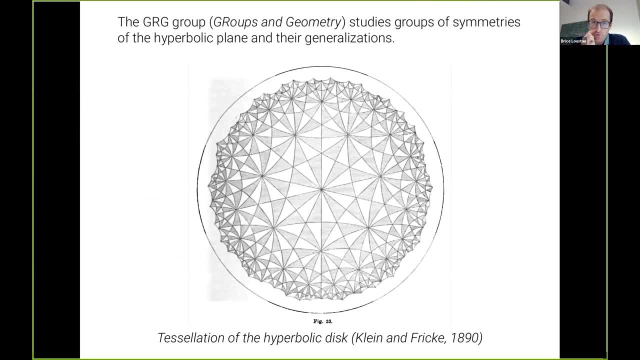 that. But let me just mention before, before I go there, that in the GRG group of Anna Wienhardt. so groups in geometry- many members, most members, are especially interested in studying groups of symmetries and groups of isometries of the hyperbolic plane and of their generalizations. 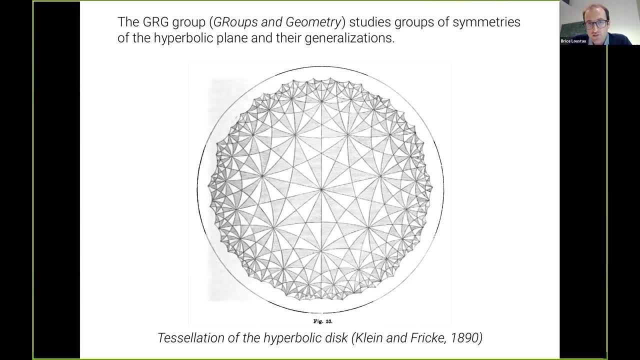 And so. so here I'm showing you on this slide what's called a tessellation of the hyperbolic plane. So this is a tessellation by triangles. that was beautiful hand drawn Drawing by Klein and Fricke in the 19th century. 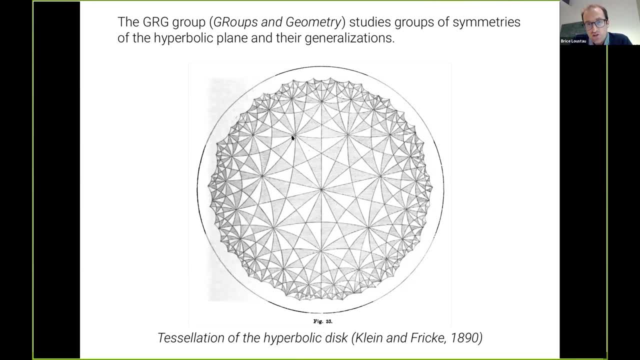 And, and so maybe you, you can see this, this tessellation has a lot of symmetries, hyperbolic symmetries, and so this, mathematically, behind this picture there is, there is a group, And it's a fascinating and rich subject to study these hyperbolic groups. 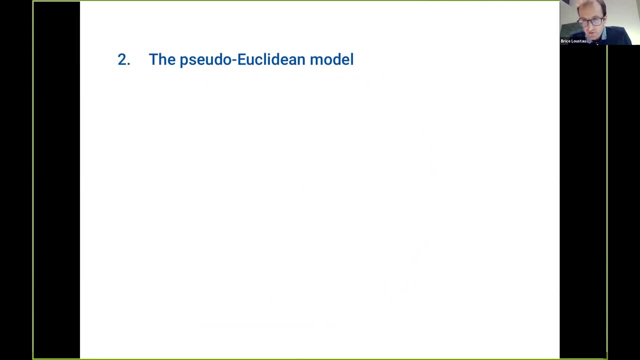 Okay, but let me move move on to the second Part, which is the pseudo-euclidean model of hyperbolic geometry and the connection to the theory of relativity. So the idea of this model is that hyperbolic geometry is anti-spherical geometry. 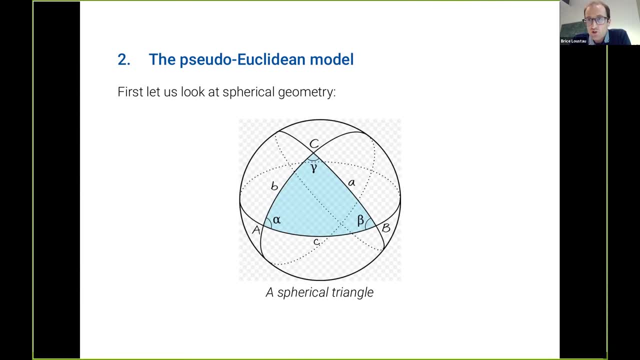 So first let us remember what is spherical geometry? Well, it's simply the geometry that you have in the sphere. So here this picture shows a sphere in three-dimensional euclidean space and, uh, it's been known for a long time that we can do geometry in the sphere. 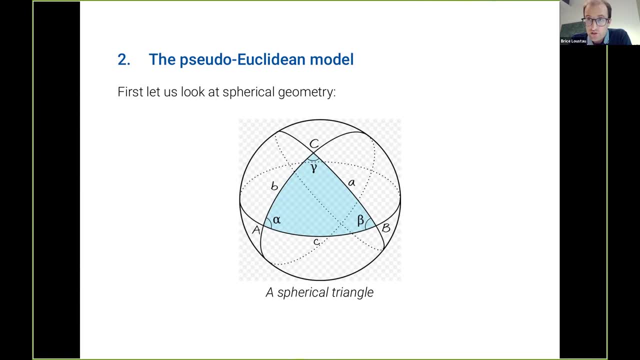 in many ways similar to euclidean geometry. So, for instance, we can draw triangles like this and we can do trigonometry and and so forth. So here, notice again that you know there's a different notion of straight line than in euclidean geometry, because you know this looks curved to euclidean eyes. these the sides of this. 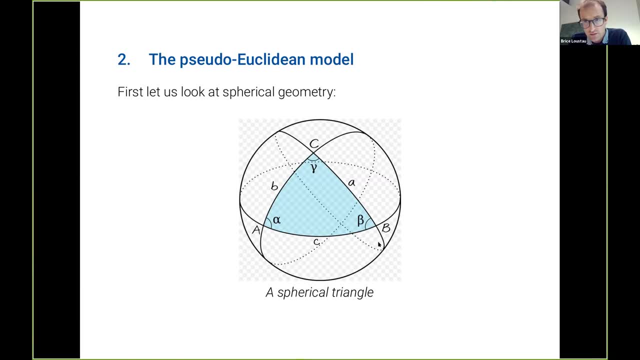 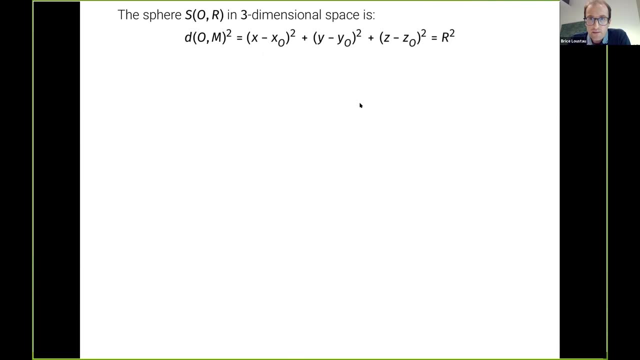 triangle, but they're straight lines, meaning geodesics on the sphere, and so those geodesics on the sphere here are great circles. Mathematically speaking, a sphere is defined as, as a set of points that are at a fixed distance from the center. So the equation of the sphere is: is this equation? 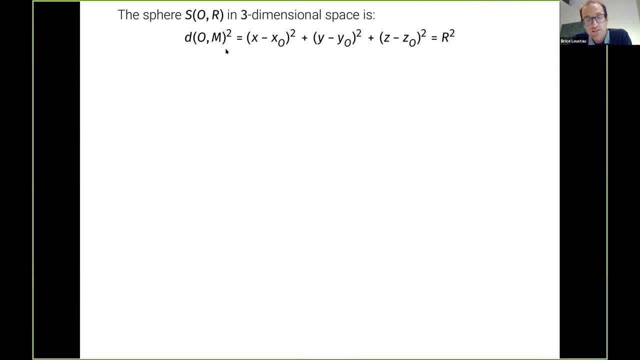 I've written here because, uh, the euclidean distance, the distance between o and m square is, is written in euclidean geometry as a sum of squares. You might remember this as a. it's a version of the Pythagorean theorem Um and here. so we're talking about the euclidean distance. so this: 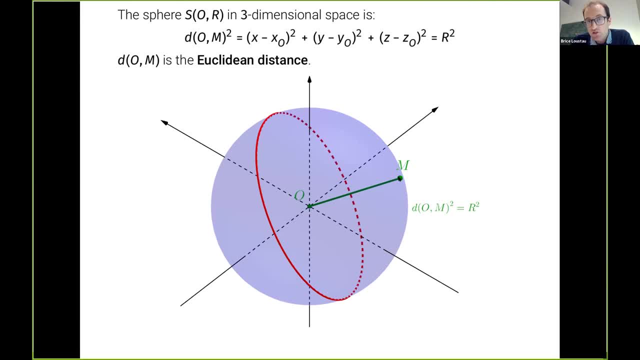 picture illustrates that if you take any point m on the sphere here, it's at a distance r from the center o, and, and so this equation that I've written simply encodes that, By definition, the curvature of the sphere is one over the radius square, which makes 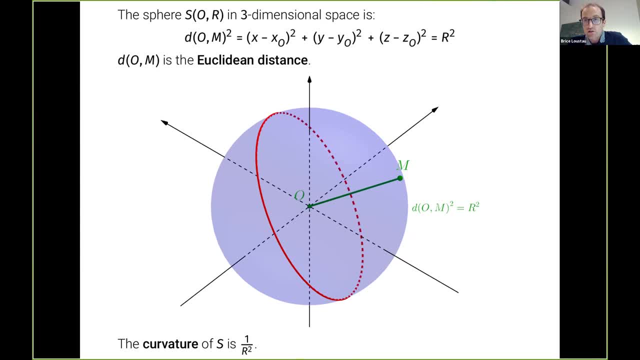 sense because it says that the bigger the radius, the the closer the curvature becomes to zero. so a very, very large sphere like the earth has a very small curvature. it's almost flat. Now what we would like to do in hyperbolic geometry is have a an analog of this with negative. 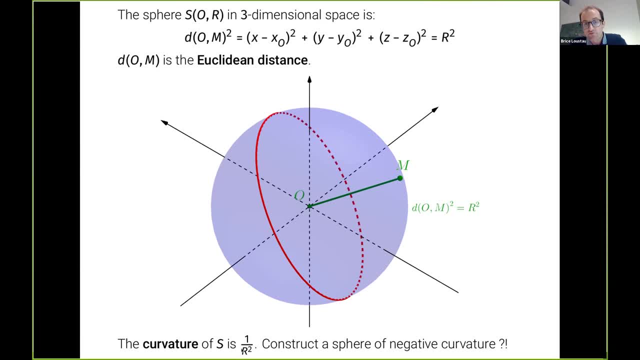 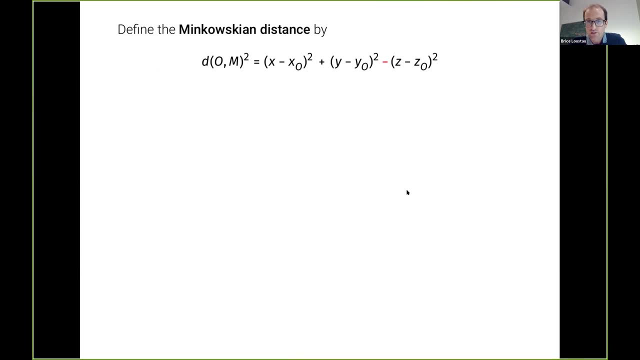 curvature, but, as you can see, this doesn't seem possible to have negative curvature, because there is a radius square here, and so that's always a positive number. So so, how do we? how do we deal with this? Well, we, we're going to define this as the minus of the euclidean, and this is where we 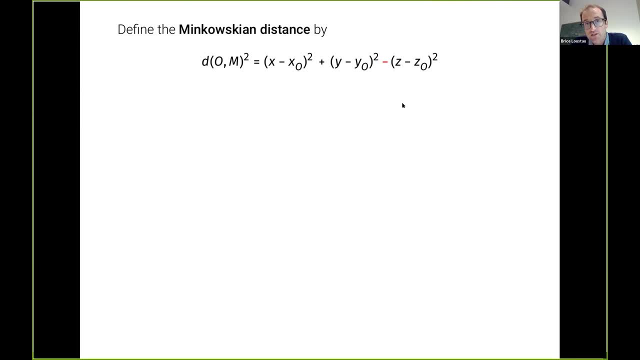 define the euclidean distance with a plus, and what we're going to do is we're going to change our euclidean distance into this minkowskian distance, where one of the plus signs has become a minus sign. So, as you can see, this was the euclidean distance with a plus, and I replace this last plus. 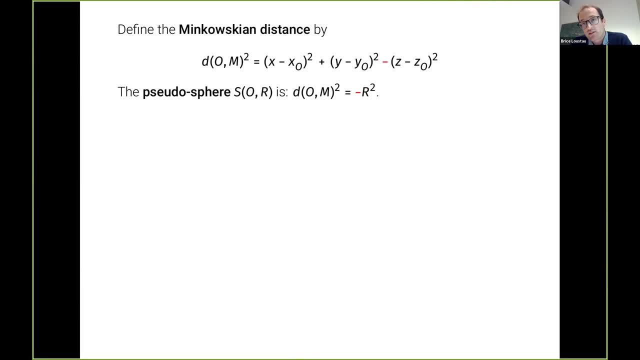 with a minus sign, and so I get something like a distance. that's a little bit weird and we call this the minkowski distance And with respect to this distance we can define. So here I put in my equation, I'm gonna put a minus sign in front of my radius square. 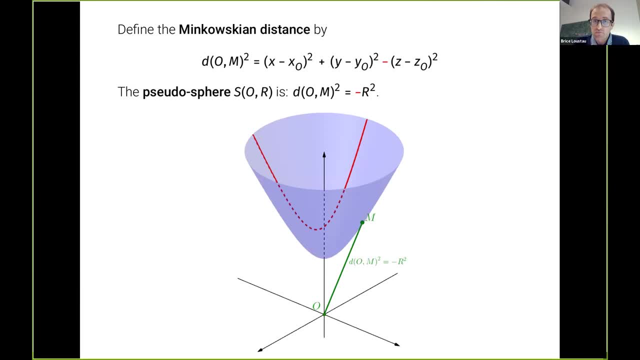 and I'm gonna get an equation of something. So if I just show you what it looks like in three-dimensional space, it's this blue surface that mathematicians called the hyperboloid. that doesn't look like a sphere at all. So this is our kind of anti-sphere. 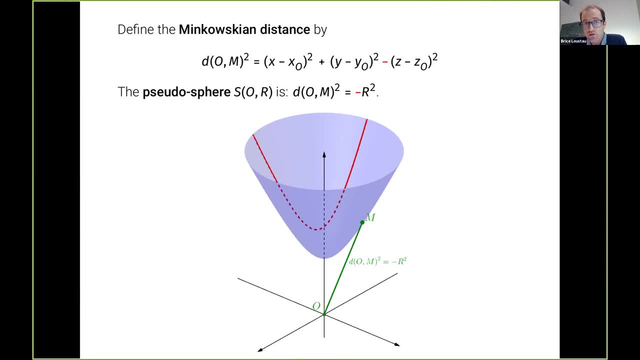 but algebraically speaking, it shares many, many properties with the regular Euclidean sphere, even though it looks completely different. I've shown you here what a straight line looks like on this surface. So it's this red line here which is the analog of a great circle on the sphere. 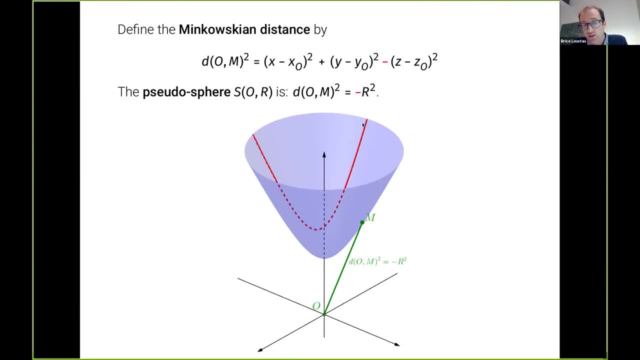 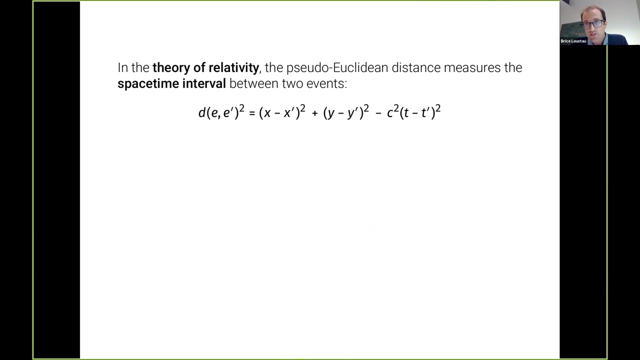 And so this will be our geodesics in hyperbolic geometry, which are hyperbolas, And this hyperbola is the reason for the name hyperbolic geometry. So the advantage of this model of hyperbolic geometry is that it makes it clear that there is a connection. 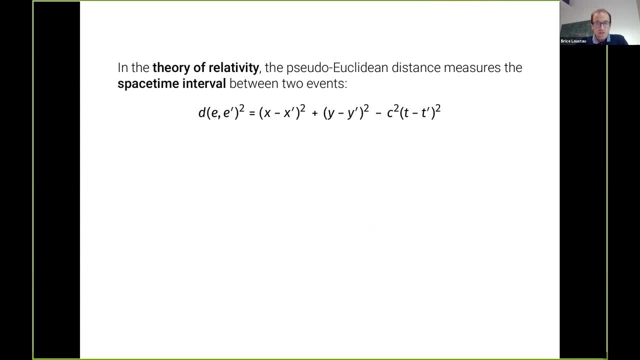 with the theory of relativity, because in the theory of relativity you have events in space-time that are represented by spatial coordinates X, Y, Z and the time coordinate T And the distance that I, this pseudo distance that I defined in the previous slide. 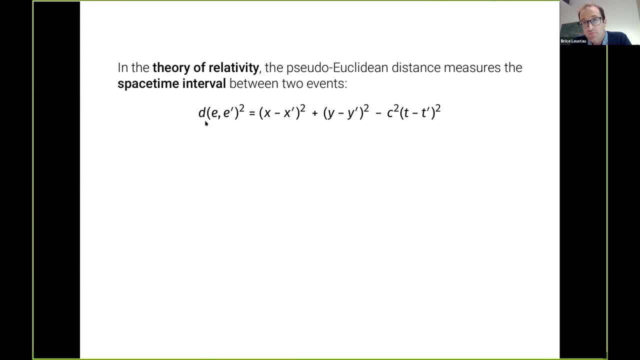 is also encountered in relativity and it's called the space-time interval between events. And this is the fundamental idea of relativity theory- is that this distance is inherent to space-time. So let me explain to you very quickly why this is the case. 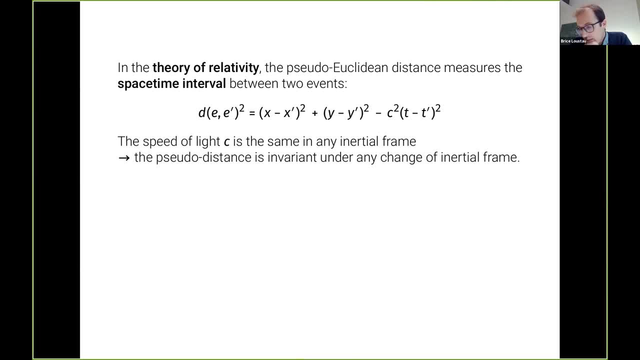 So theory of relativity was developed after people realized experimentally that the speed of light is constant in any referential, in any inertial frame, which violates Galilean physics. You know, in Galilean physics, when you change observer, 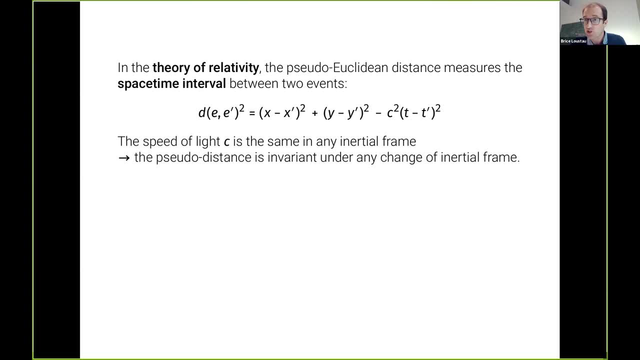 you have to add the velocity between the two observers to the velocity of an object, And so the velocity of an object can be, the speed of an object can be infinite. But here we observe that the speed of light is just doesn't depend on the referential. 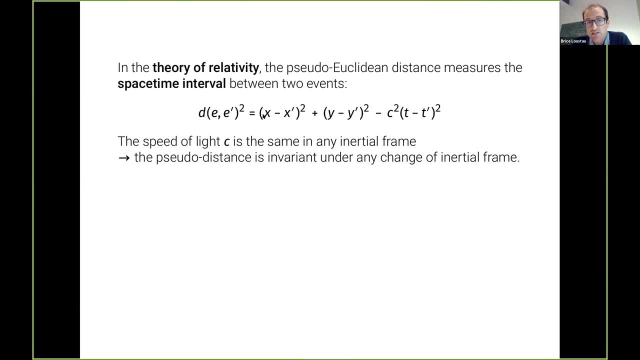 And mathematically it's easy to show that this means that this pseudo distance I've written here is invariant when you change your inertial frame, when you change the observer. And so, because of this same pseudo distance in hyperbolic geometry, 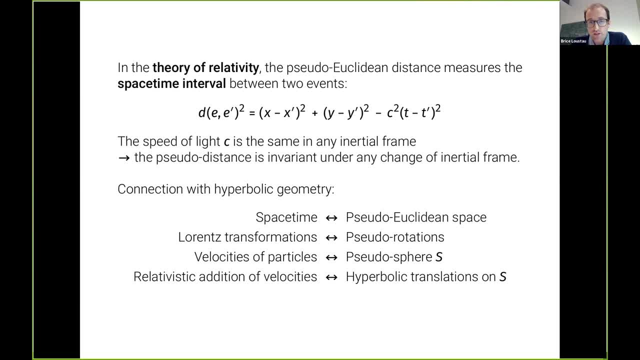 there is a kind of dictionary between hyperbolic geometry and the theory of relativity. So, for instance, the change of observers, the change of inertial frame, in physics are called Lorentz transformations and they correspond to pseudo rotations, meaning rotations of our pseudo-Euclidean space. 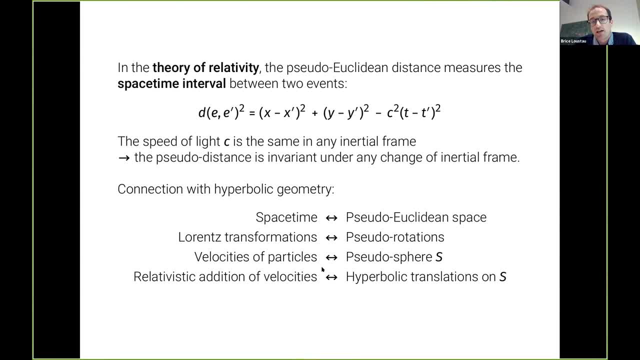 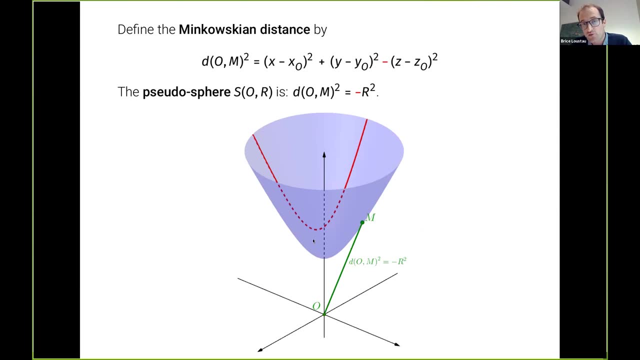 in hyperbolic geometry And in physics the velocities of particles correspond exactly to points on our pseudo-sphere. So, if I should, okay, if we go back to this. so this blue surface is our hyperbolic space and points on this thing represent velocities of particles. 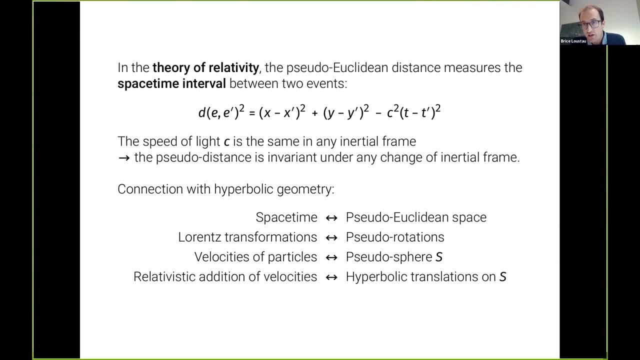 So in physics, instead of the Galilean way to add velocities of objects, there's a different way that you add velocities, which is this famous relativistic addition. So there is a formula that I'm not writing which tells you when you change observers. 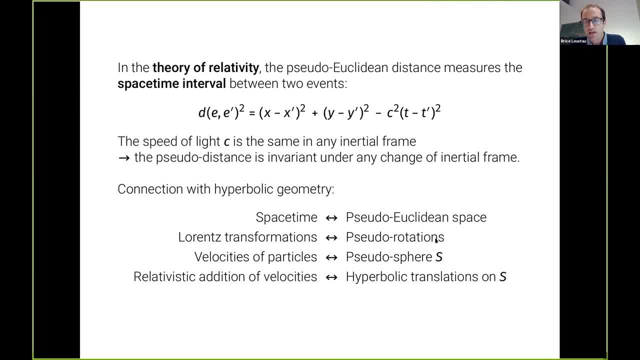 how you add the velocities of particles, And in hyperbolic geometry, this is a very simple geometric transformation called the hyperbolic translation, And so I'm going to use this- I'm just not telling you this for no reason- in my final section. 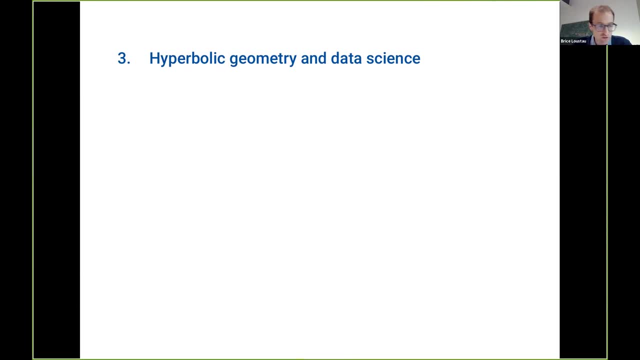 which is the application of hyperbolic geometry to data science. So first let me quickly define a few terms if maybe you've never heard of data science before. So one could define it as the science of extracting information from data And one crucial question for this. 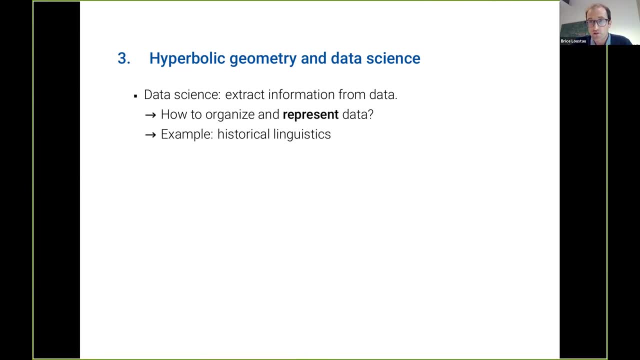 is how to represent the data that you're given in a way that makes it best to analyze it. Machine learning is a closely related field, where the idea is that it's a way to develop algorithms that can learn with experience, And so the more you feed machine learning algorithm data. 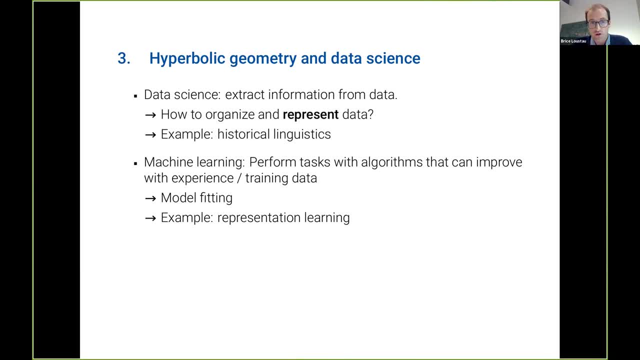 the better it becomes, And this can be especially useful for what's called representation learning, which is this, solving this question of how to represent the data. And a subfield of machine learning is deep learning, where the main player is these deep neural networks. 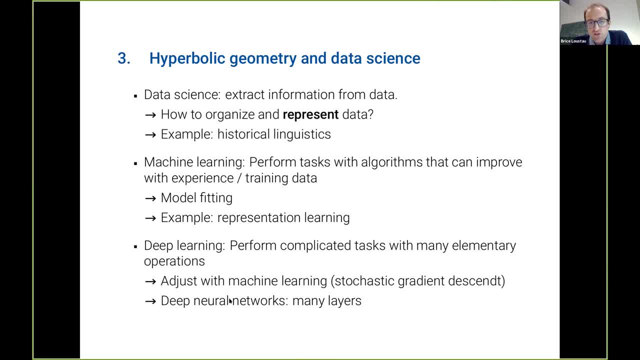 And the idea here is to develop machine learning algorithms that are just the representation of the data. It's the repetition of many, many, many elementary tests And you adjust these algorithms. So these algorithms have many, many parameters and you adjust them with training. 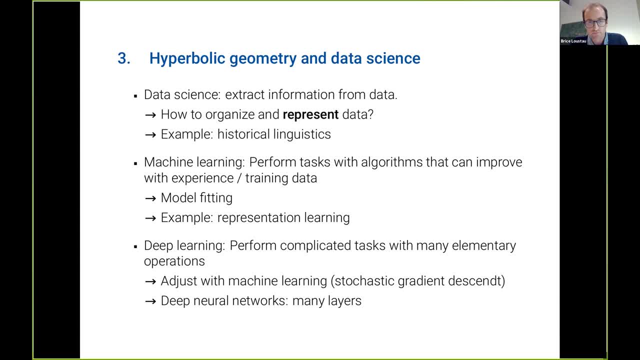 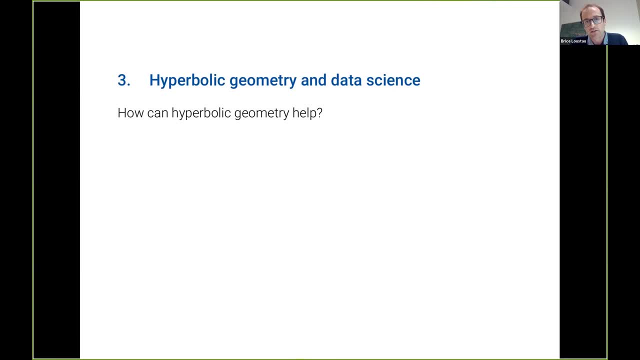 So with experience. mathematically that's a gradient descent method. So I'm going to say a little more about all of this, but first let me motivate. So why can I want to make the point that hyperbolic geometry can be useful? 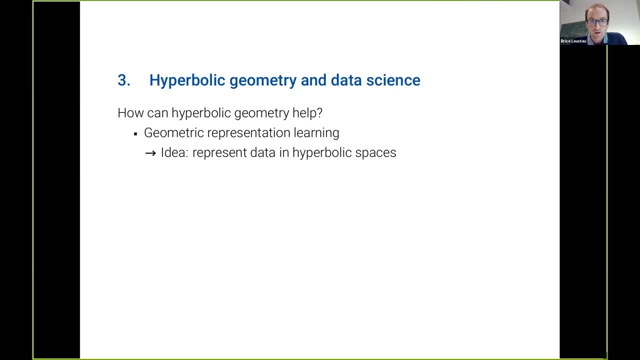 For this. and so what is the idea? Well, there's two things. First of all, there's the idea that for representation of the data, so for representation learning, it might be a good idea to represent our data in a hyperbolic space instead of a Euclidean space. 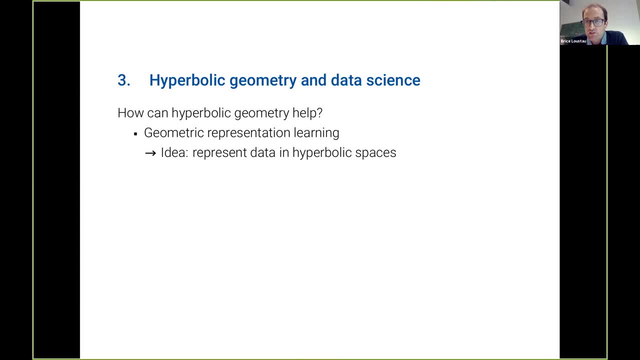 So you know, usually, typically, you would represent data, for instance as a graph, embedding in a Euclidean space, meaning you kind of draw a cloud of, or nodes of, edges and stuff and maybe a two-dimensional or a three-dimensional or a higher dimensional space. 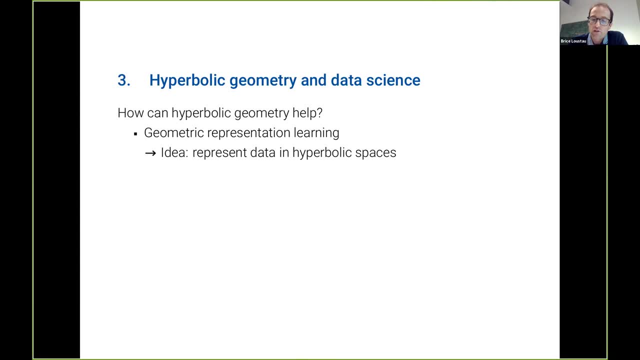 but it's always kind of a Euclidean space And one could think about doing a similar thing in the hyperbolic space. And the second idea where you can use hyperbolic geometry is so this field called geometric deep learning, where we're going to define 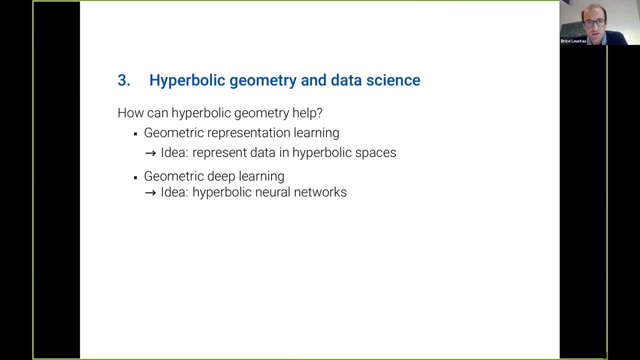 some kind of hyperbolic version of neural networks, and I'll say more about that, about that. So why is this a good idea? Why would anyone want to do this? Well, it so happens that many data sets in a way have an inherent hyperbolic structure. 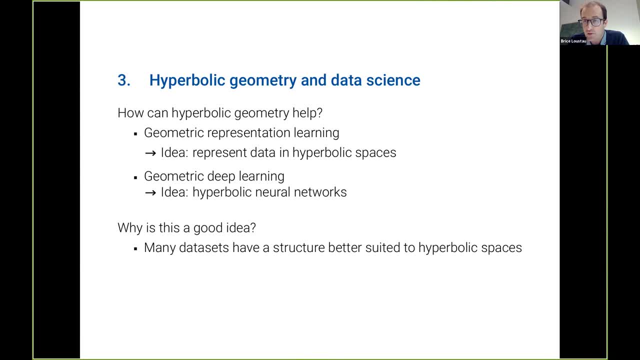 And so many data sets are best represented in hyperbolic spaces, And I'll try to tell you why. And so, in particular for these data sets, it makes sense that you would adapt your machine learning algorithms to reflect this geometry in their architecture. 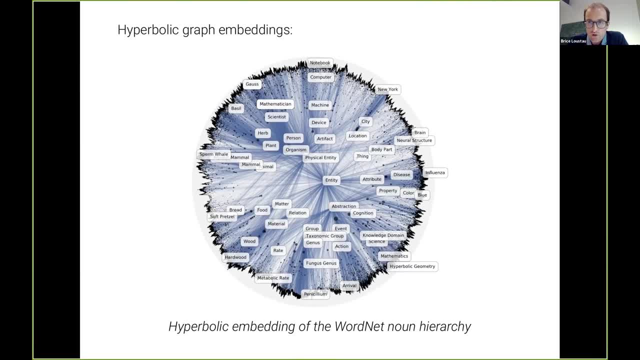 Okay, so I'll finish by explaining a little bit more of what I mean by all of this. So this is an example of a hyperbolic graph embedding for the data set called the word-net-noun hierarchy. So you see, this data set consists of many, many words. 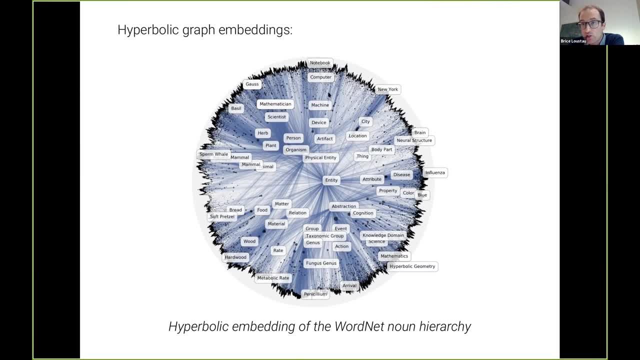 many, many nouns, and there's a hierarchical structure. Nouns are related by semantics, They can be synonyms or super-nonyms or whatever, And so you can represent this kind of as a graph structure, And so this picture shows an embedding of this data set. 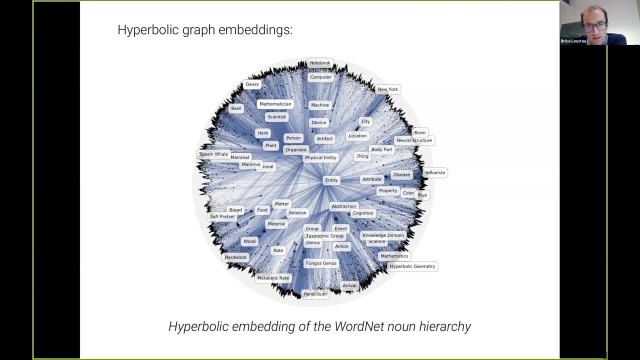 in a hyperbolic disk, And so you might notice that like there's these dark areas near the border, So it looks so this means that like there is an unbelievable amount of nodes that are compressed near the boundary. But you have to remember that. 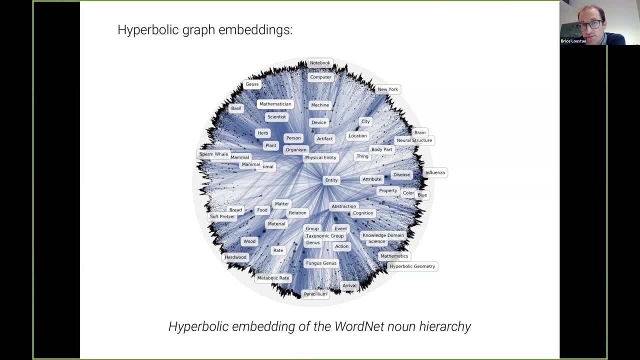 so this is not a flaw of the embedding, but this is a feature of this model: that distances are compressed when you approach the boundary. So it's not a flaw of representation. but if we had a hyperbolic eyes, we would see all this data nicely spread out. 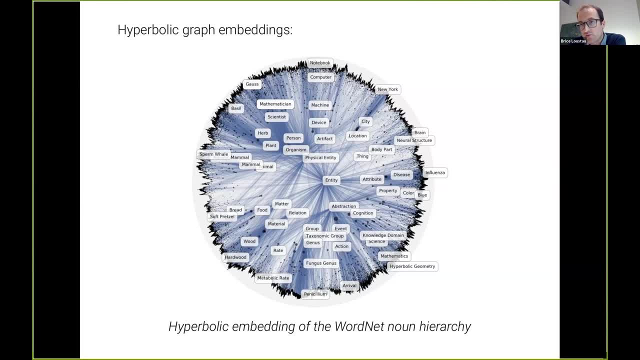 in this hyperbolic disk And it's not possible to nicely spread out all this data in the Euclidean model. And the reason is because this data set has this inherent hyperbolic structure set differently. There is kind of an exponential growth to the number of nodes. 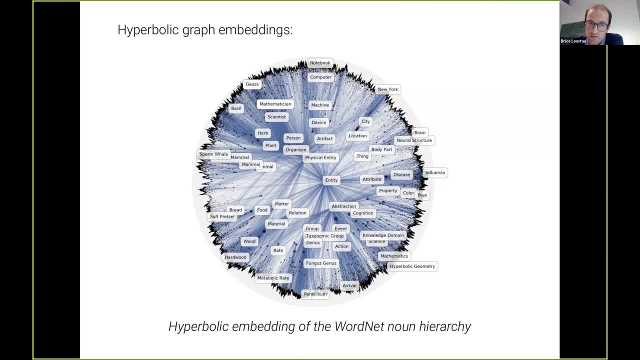 So you start from one node: it has many neighbors, and each neighbor has many neighbors and you have, you know, you have- a kind of exponential growth rate, And this happens a lot for many data sets And these data sets are best represented. 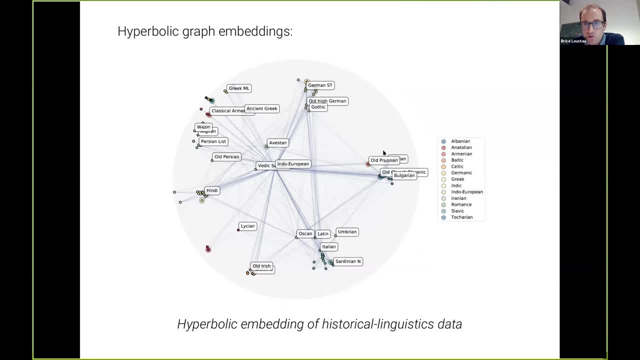 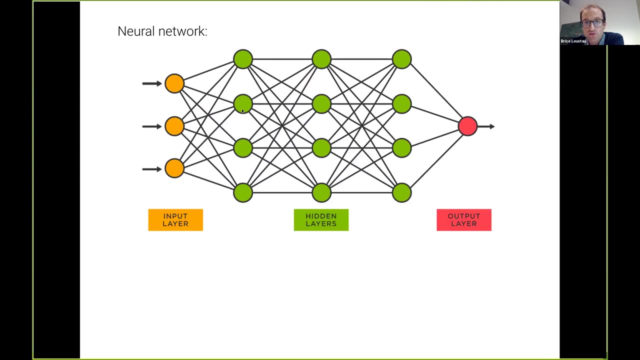 in the hyperbolic space. So here is just a second similar example with historical linguistics, so where nodes are ancient languages and you have hierarchical relations between them, And so in order to solve these tasks and do these representations, one might try to do some hyperbolic version of Debron. 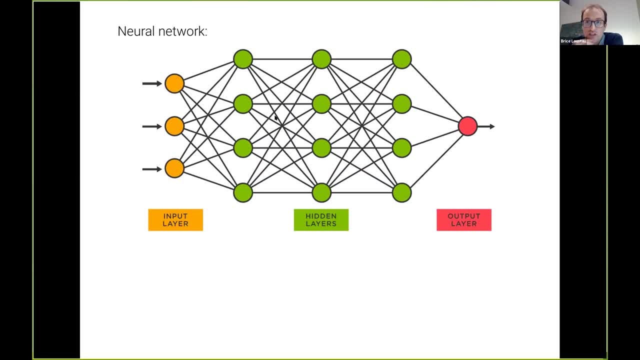 that's a new kind ofOLLine, And what this means is you. you take a standard neural network, So if you've never seen one, it looks kind of like this diagram. So neural network consists of mini neurons that are organized in layers. 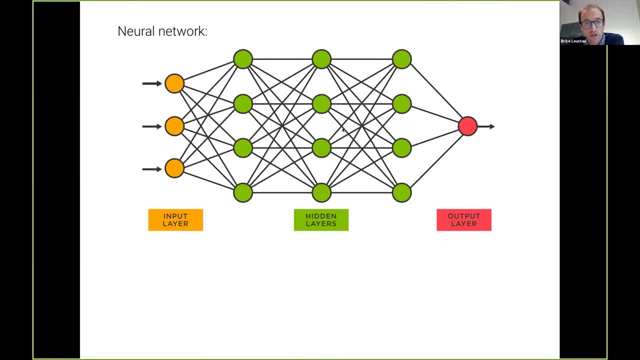 and each neuron performs very simple operation. So typically you have the input layer, So these first orange neurons- they take some data- and then you have these many hidden layers that apply elementary operations with parallel network And you sort of punch them into a good way. 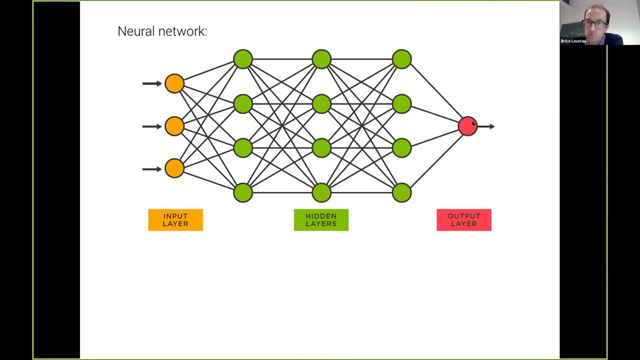 Thanks, guys, for questions or any other stuff. I'll see you in the next session everyone. Thank you so much. See you again. parameters that you have to adjust And then finally, you have this alpha layer that gives you the results. 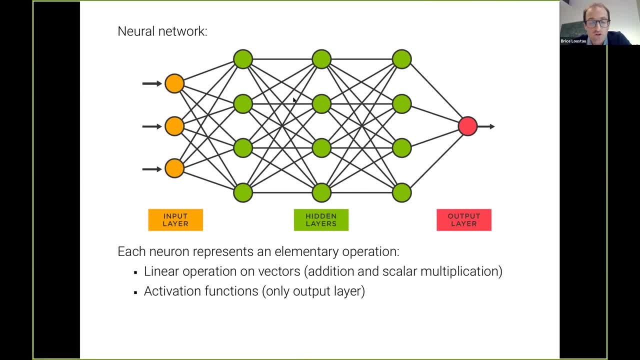 And these elementary operations are almost all of them are linear operations of vectors, such as the addition of vector or the scalar multiplication of vector value constants. So this is what all of these green neurons operate, And typically you also have activation functions in the upper layer, but let me kind of ignore this. 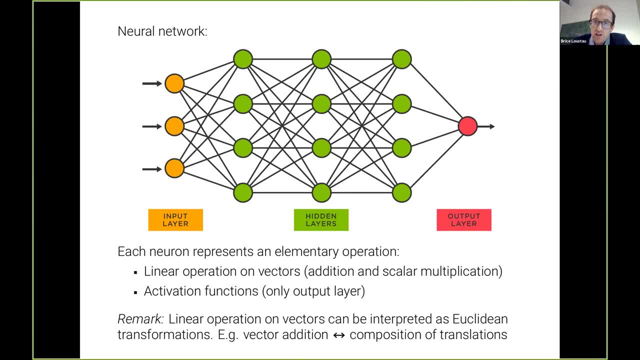 Now the essential idea is that these linear operations- there is a geometric interpretation of them as Euclidean transformations. So, for instance, a linear addition of vector. you can think of it as so: adding a vector is like translation in the Euclidean space. 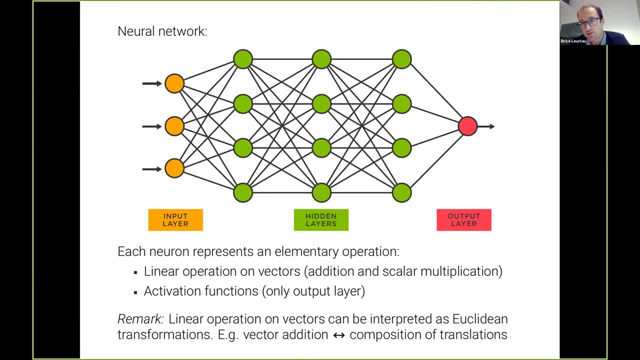 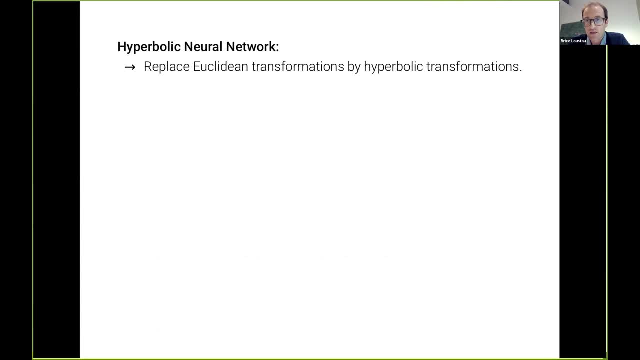 And when you compose these operations- adding and adding- it's like composing translations, And so, in a way, we're talking about Euclidean transformations of our data set, And so when you see things like this, it's clear what the hyperbolic version of this should be. 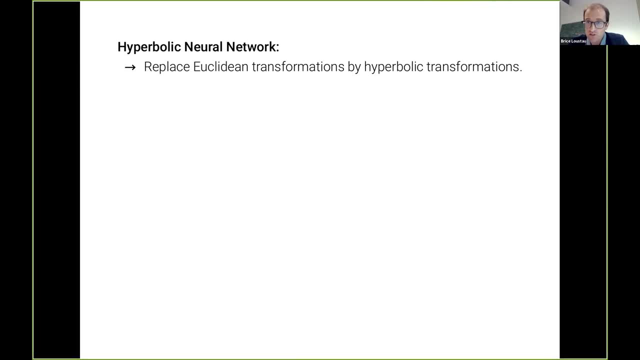 It's applying hyperbolic transformations, hyperbolic geometry transformations, instead of Euclidean transformations, So in particular, these hyperbolic translations I mentioned before. But the cool thing is that, as I've mentioned before, this hyperbolic translation is nothing else. 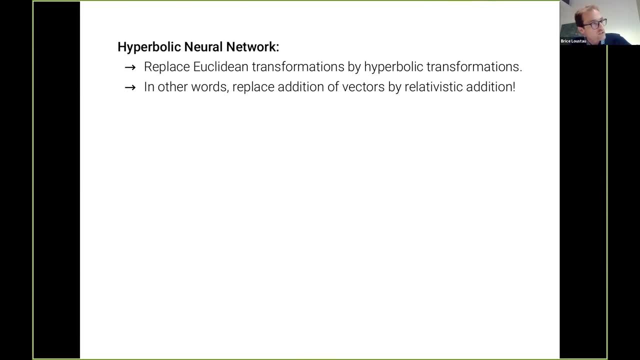 than the relativistic addition of velocities, And so this puts it in a this way. to put it, this way to put things, it makes it kind of practical for people to code, For instance, where you take your standard neural network and all you do is you replace the standard addition. 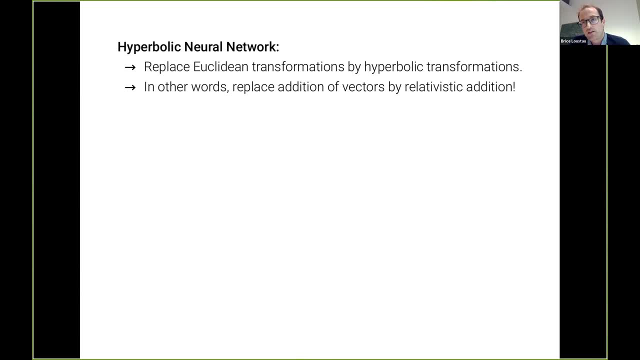 by relativistic addition, and you can find the formula in any book, And so this is a relatively new field, this hyperbolic neural networks and geometric learning- But my understanding is so far, empirically speaking, it works. there's good results of how this works. 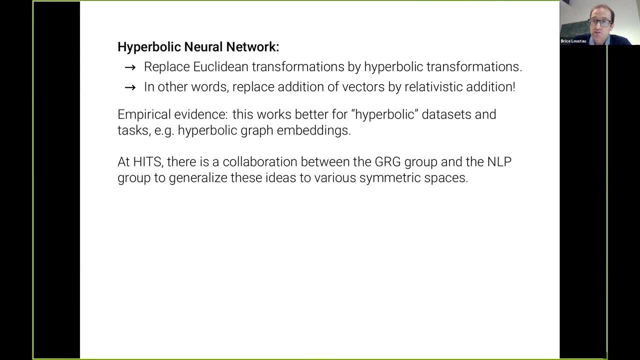 And I'll finish by mentioning that at HITS there's a ongoing collaboration with members of the GRG group, And so the math group and the natural language processing group, to generalize these ideas to more general geometric spaces than hyperbolic spaces, that are known as symmetric spaces. 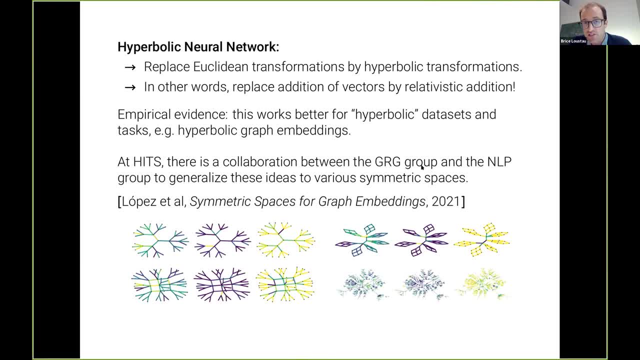 So, for instance, there's this paper, Symmetric Spaces for Graph Embeddings, by Federico Lopez And Naveen Hardin and others who study graph embedding, the graph embeddings in symmetric spaces. All right, thank you very much. Thank you so much, Ries. 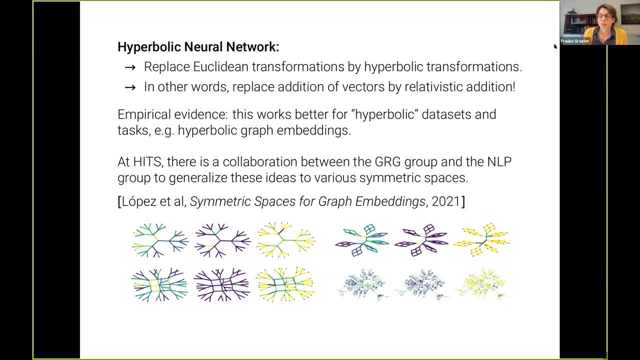 for this really excellent talk. Brilliant. The discussion is open. I welcome questions. It was very approachable for the non-math people. I would say so go ahead. No boundary circle questions. yeah Yeah, thank you very much for this fascinating talk. 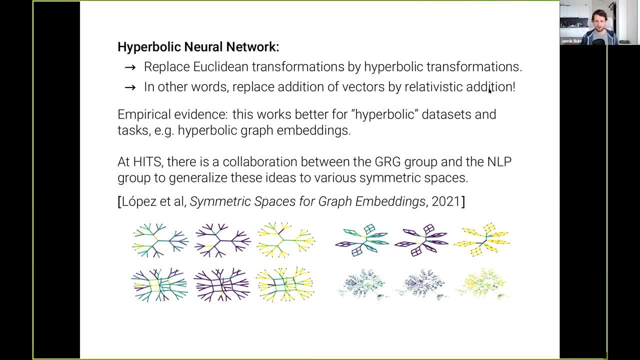 I think it's very fascinating topic and really mind-bending. Are there any ways in which you can like, for example, in multidimensions? Euclidean space is already really hard to wrap your mind around, but is it even possible in how you study this in Helium? 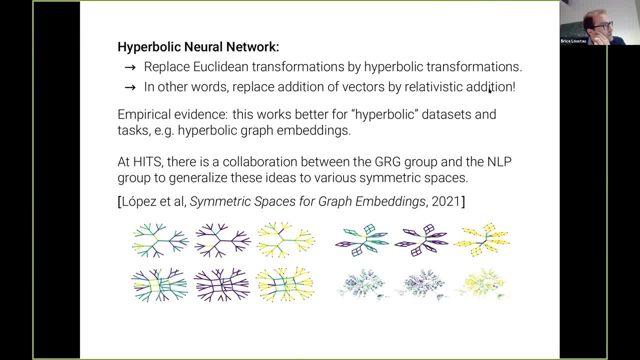 even possible in hyperbolic space, Right? So yeah, so that's a good question, And high dimensionality is a thing that's very important in data science, And the key question is: typically: you start with data that is represented in many, many dimensions. 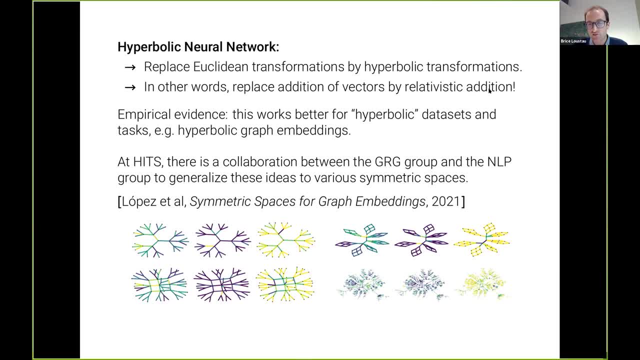 And what your neural network's task is. a lot of the time is to try to reduce the number of dimensions. So it's true that high dimensions are hard to wrap around your head around, But it's not hard actually for computers And for computers, linear operations. 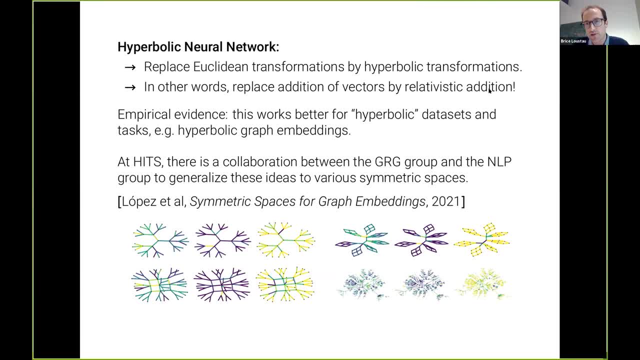 they don't care that it's three-dimensional For us. ooh, what's four dimensions? It's complicated, But for computers really, it doesn't make a difference. And computers more and more. the architecture is especially designed, like these GPUs and so forth. 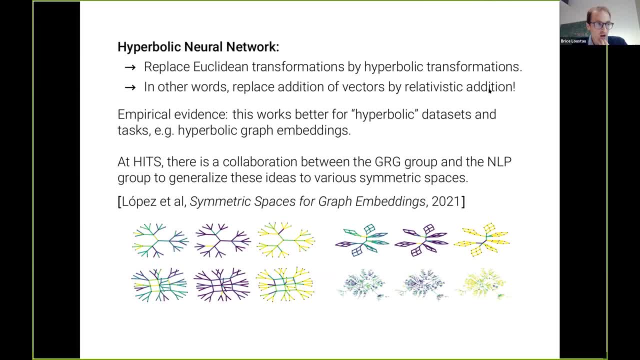 to handle these linear operations Now. so hyperbolic geometry, I would say. for mathematicians it's also not a big deal to have high-dimensional hyperbolic spaces. It's not something you just get used to. You can't really see them, but they're not that mysterious. 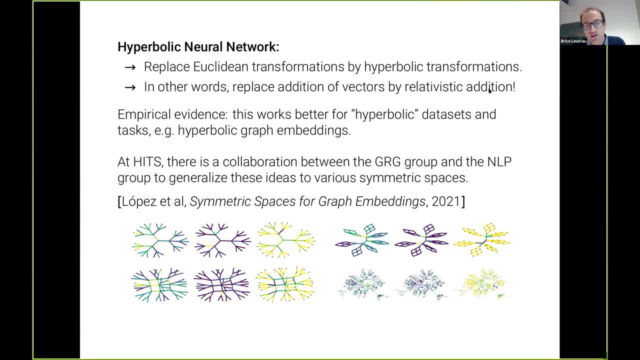 Now, on the other hand, I think what's true is that computers are not well-adapted to deal with hyperbolic geometry and hyperbolic operations, And that's, I think, probably one of the big limits of geometric learning is performance. 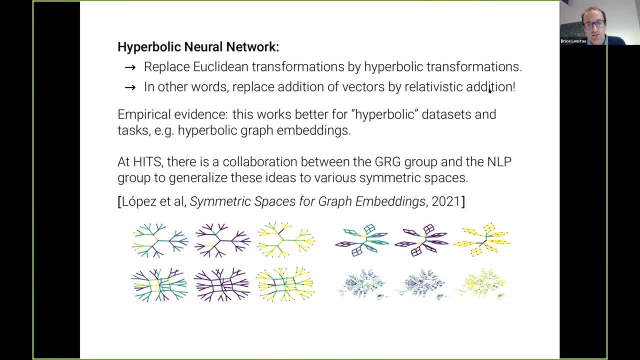 So I'm really not an expert, but I think theoretically speaking, geometric learning can be much more efficient than standard Euclidean. But then in terms of processing computer time it's probably kind of tricky. Thanks, Saskia. Who's next? 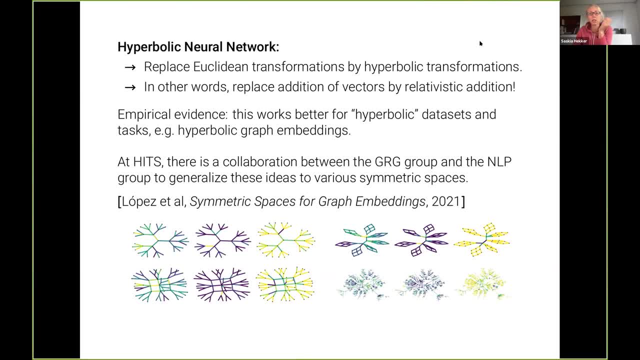 Thank you very much for this very nice talk. I have just one question. So you say that a lot of people don't know how to do it. How do you do it? A lot of data sets are hyperbolic, But how can you easily test whether or not? 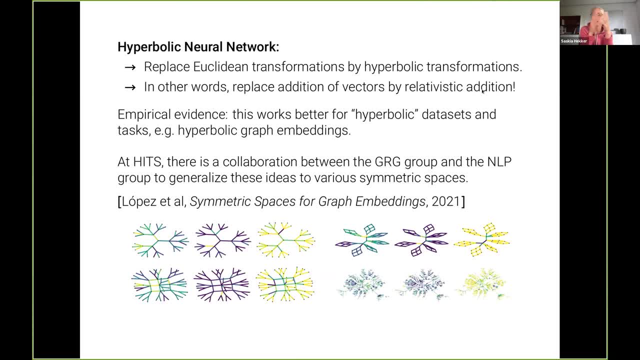 your data set would fit better on a Euclidean space or on a hyperbolic space? Yeah, that's an excellent question And I think this question is basically a lot of what the research is about, And it's not necessarily easy to answer. 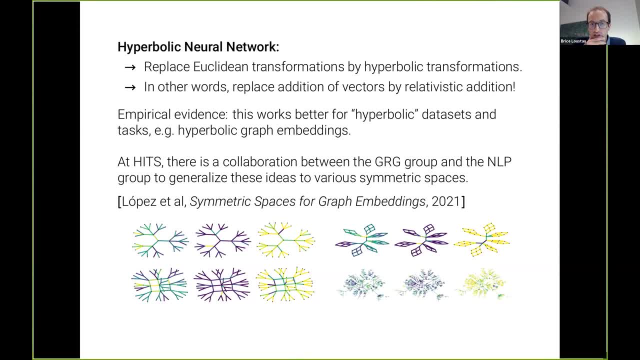 And in fact so you could even extend this question to like. well, maybe not all data sets are Euclidean or hyperbolic. Maybe some of them have an inherent structure that are, So for example, you could imagine a data set that: 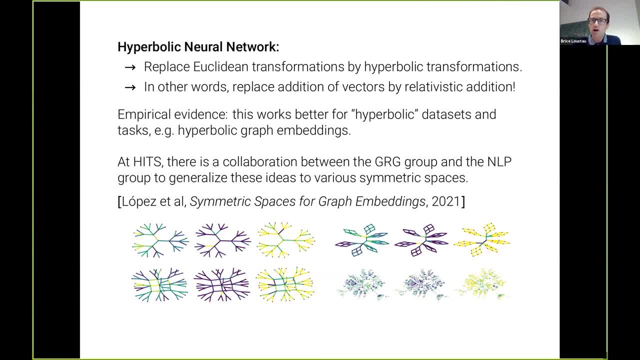 is a mix. It's partly Euclidean, partly hyperbolic, And so how can you predict this in advance, Like what is the best way to represent your data set, And so I'm not part of this collaboration, And some of the authors are here listening. 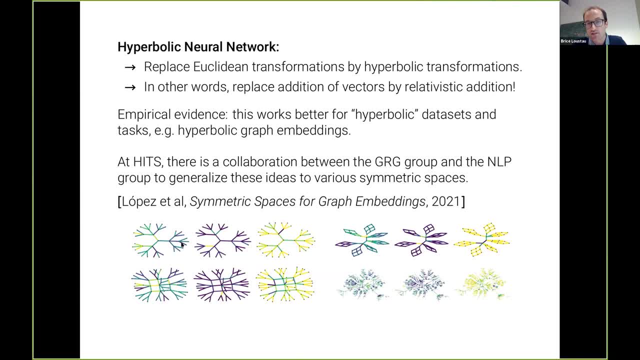 But I think that's a good question And I think that's partly what they address in this paper. So you see these graphs here that I've shown that you see on this slide They try to represent them into different symmetric spaces and see which ones get the better embedding. 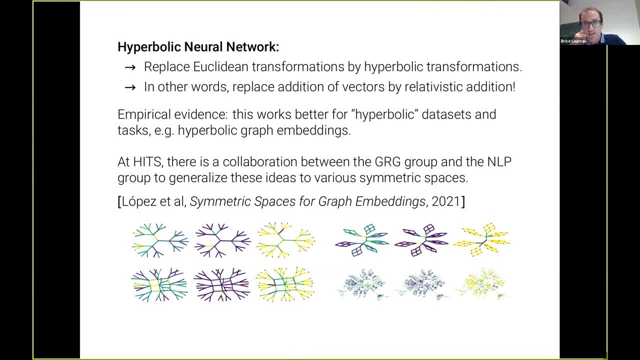 What I would say is that you could say that in some sense you could expect hyperbolic data sets to be generic. It's kind of surprising. So if I give you random data sets, I would probably predict that it will be hyperbolic and not Euclidean and not anything. 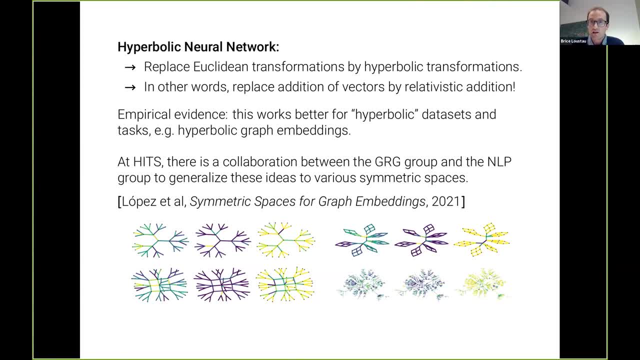 And that's just because of this phenomenon that I briefly mentioned, that basically, graphs typically have an exponential growth. So, for instance, if you do, I don't know, like a genealogy tree where each generation has n children, then very quickly you'll see an exponential growth rate. 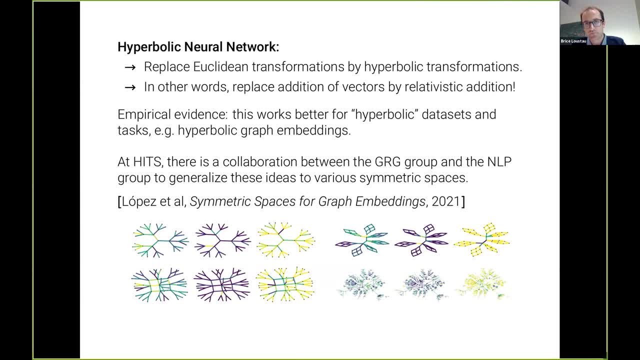 And that's kind of a characteristic of hyperbolic, It's not a geometry. OK, thank you very much. Thanks, Camilo has got a question. Yeah, Bryce, thank you very much for this very nice presentation. I had a very simple question. 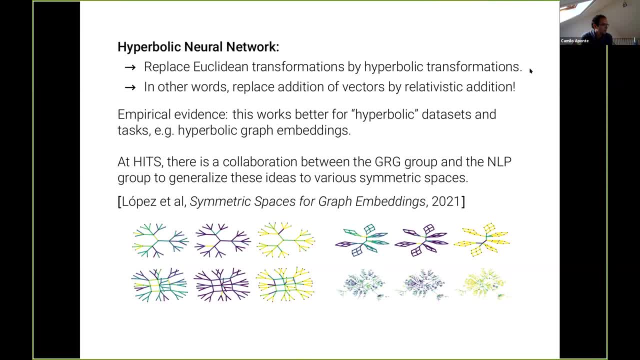 I was wondering whether the hyperbolic or the Euclidean neural networks give a different result, And the difference is more how you handle the data internally to get that same result, or it's actually two very different outcomes? And if it's two different outcomes, 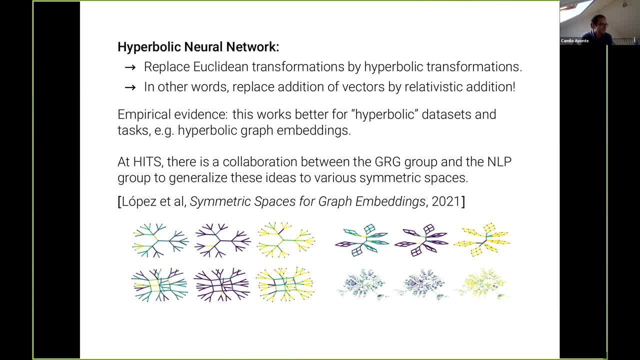 how do you judge whether it's an Euclidean or a hyperbolic representation? the best way to go, Right? Yeah, that's a very good question And, to be honest, we're reaching the limit of my expertise. You know I've not dealt that much myself with 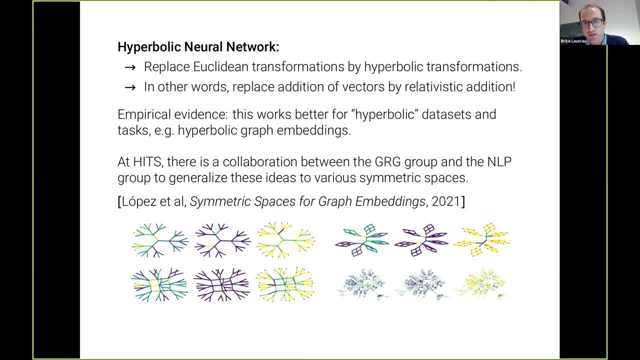 Hyperbolic neural networks, hyperbolic and otherwise. So some people here would give you a better answer than me. But first of all, you know it's not an obvious question. It's like how you have to set So typically when you do machine learning. 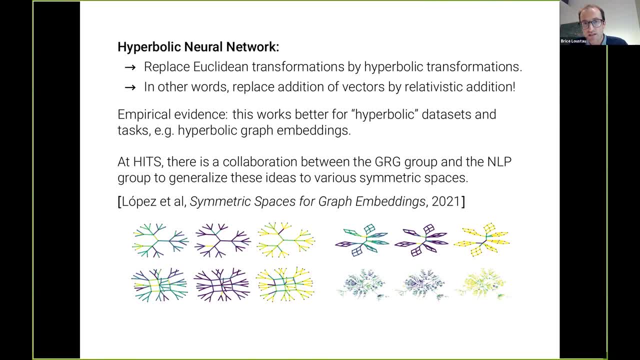 you have something like a cost function, something that you want to optimize And that's supposed to measure. So the answer also depends on if you know in advance what you want to optimize and how you want to measure it. OK, And so, for example, you know a typical example. 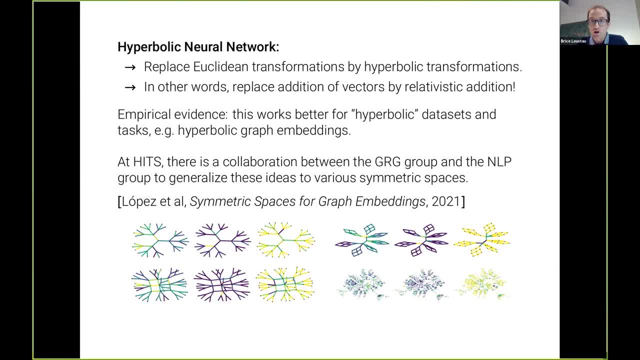 in machine learning, I think, is this notion of autoencoder, where you have a bunch of data, you force it into a model and then, with machine learning, you try to see if you can recover the original data, the features of the original data that you started from. 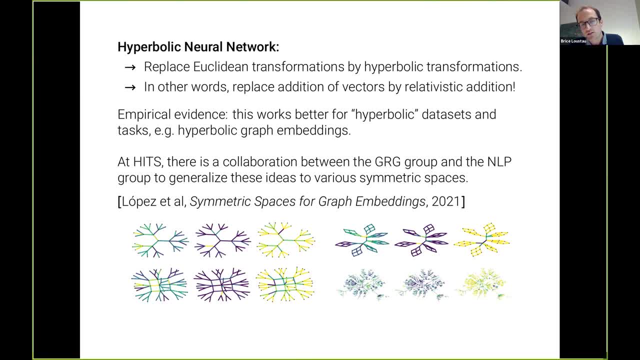 And so this is some way you can test if your algorithm is doing a good job or not. But yeah, So certainly I think it's. an important part of the question is how to measure the effectiveness of these machine learning algorithms. If I may still ask one question, because you 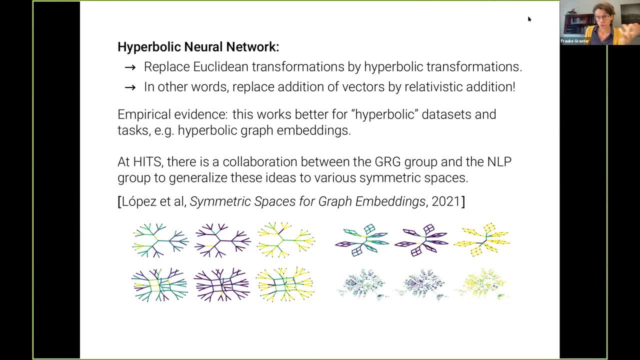 said it is open. what really fits better to the hyperbolic space or not, or Euclidean space? Yeah, Yeah, Yeah, And that is, are all of these social networks or traffic networks, graphs that many have looked in, and often they're depth-scale free. 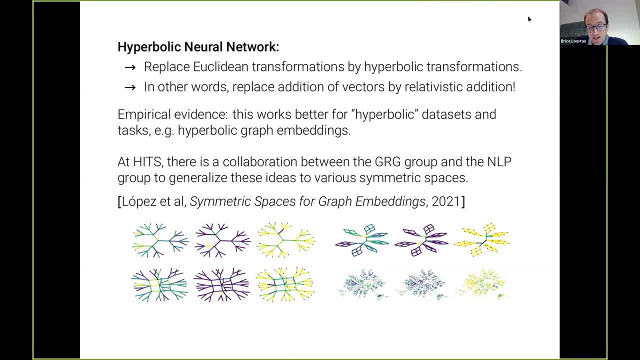 would they fit really well into this hyperbolic geometry, such data, Yeah, I mean, I don't know the answer to this. I think it's still ongoing research And so people are studying this. What I can tell you is that when I prepared for this talk, 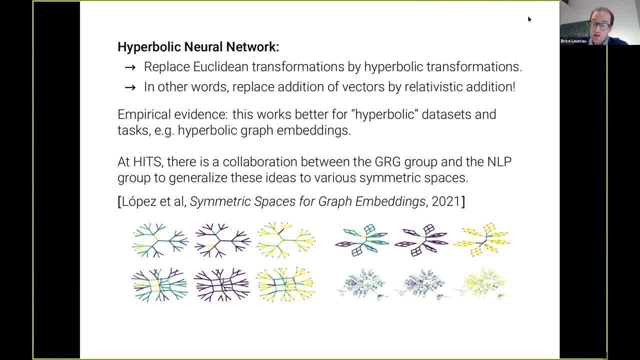 you know, superficially, like I Googled, you know, geometric deep learning to see what's going on and, for instance, i i found a blog post on the internet that was on geometric deep learning. that was written by a facebook- uh, a facebook engineer. so and and so and they're saying: oh, it's a new. you know, we're all changing.